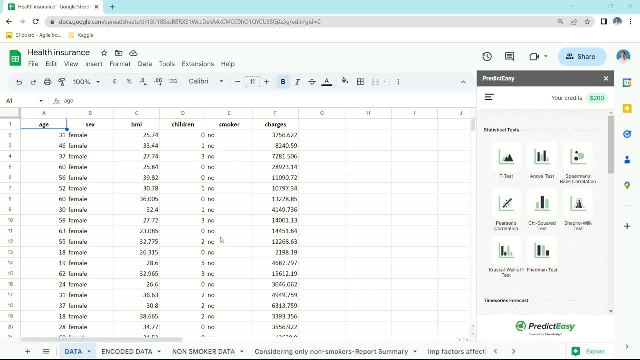 And this is the data set we'll be taking today for use case. I've already encoded the data because we all know that machines will understand numbers better than words. As per usual, we have already framed three simple questions. Let's see how we can find answers using Predict DC. 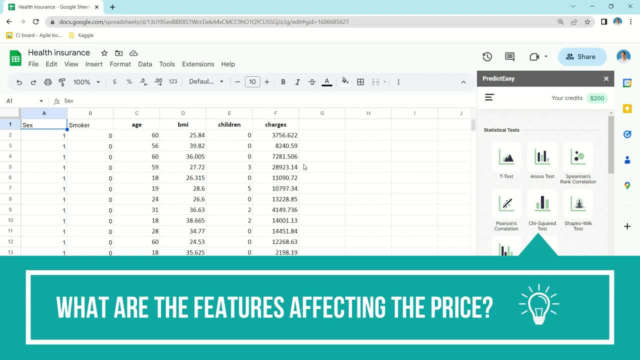 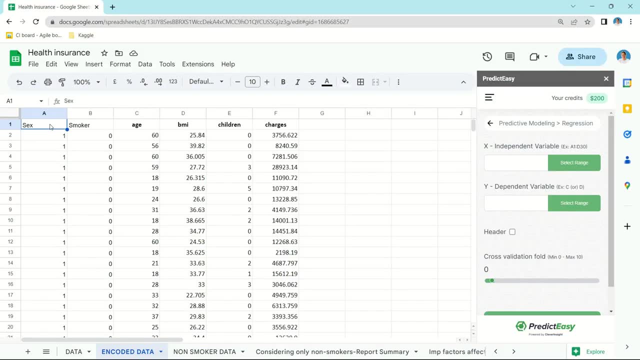 First one: what are the features affecting the price? To find the answer, let's carry out the regression test. Let me select the independent and dependent features here, And I'm also selecting the header checkbox because we are including all the headers from the data set, And I'm also setting the cross-validation fold to 2,. 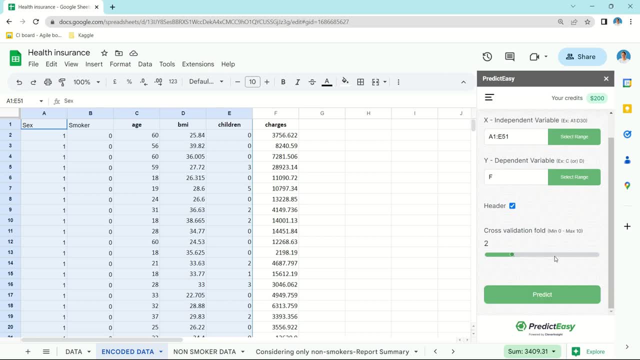 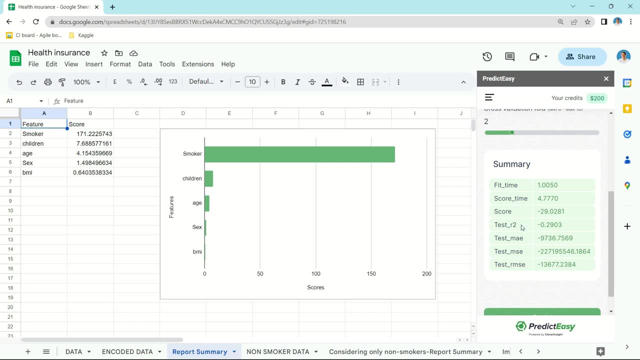 which means 20% of the data will be used to test the model. Let me click on predict. We got the summary. We can see the result of R squared mean average error, mean squared error and root mean squared error. So these values will be able to evaluate the model as a fold. 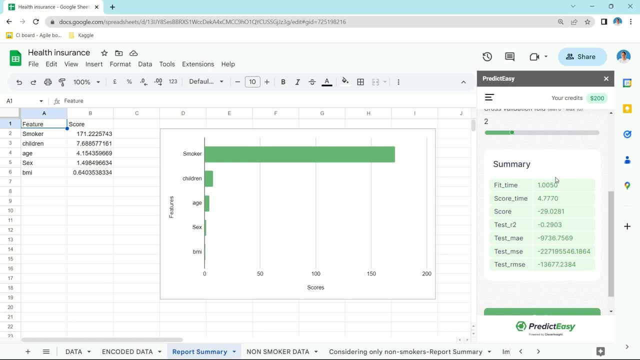 whether the model is something reliable or not. So, according to the question, Predict DC has come up with some important features in the graphical format. So we could see the top three important factors which will help us predict the prices: whether the client is a smoker or not, the number of children the client has and also their age. 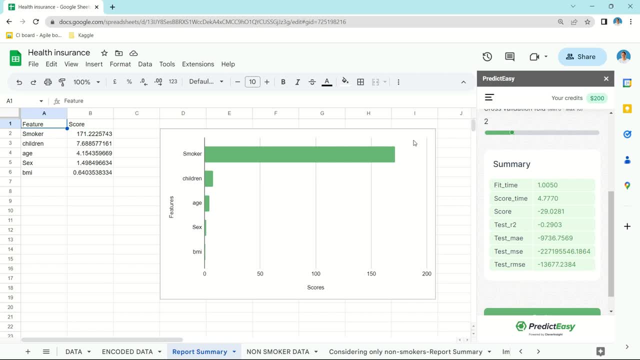 The beauty of this tool is that the user need not write even a single line of code because it is a no-code platform. So this is a major difference between the traditional way of analyzing data and analyzing using predict EC. I mean, it is very user-friendly: with just click a few buttons you'll be able to get results. 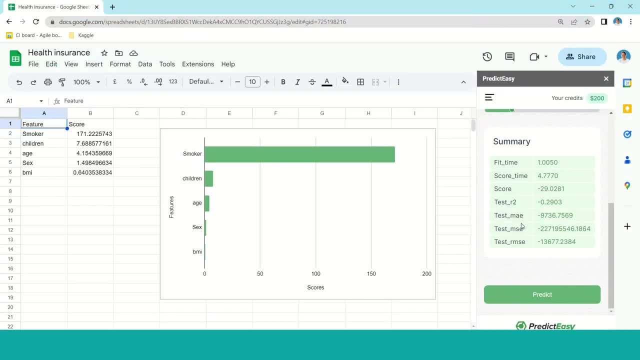 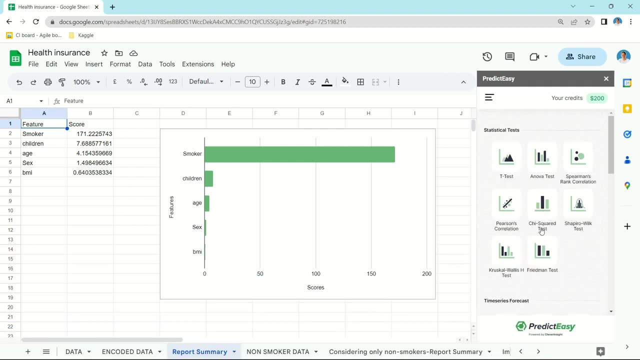 Moving on to the next question, let's check the BMI feature, whether it is distributed evenly or not. For this, let's carry out the Shapiro Wilk Test. So this is a statistical test which will help us understand whether the data is spread gaussianly or not, That is, whether the